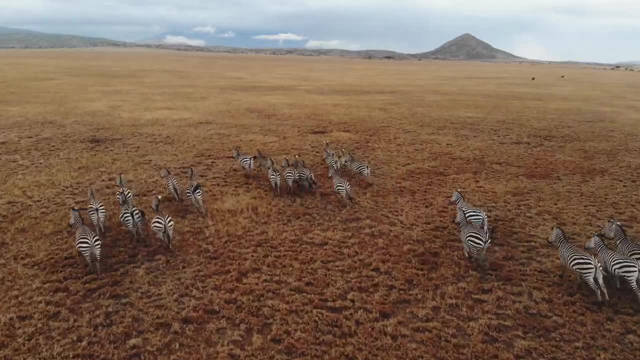 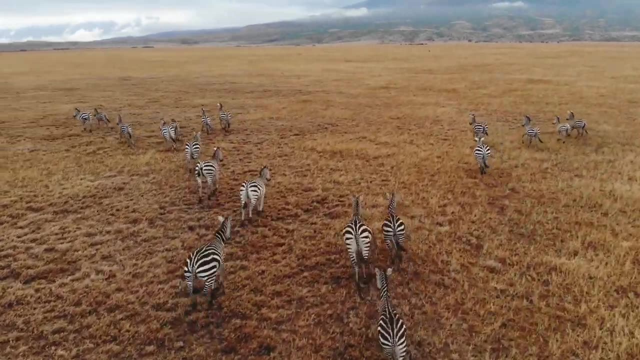 them use this large size to their advantage. When all the zebras keep together as a big group, the pattern of each zebra's stripes blends in with the stripes of the zebras around it. This is confusing to the lion, who sees a large moving striped mass instead of many. 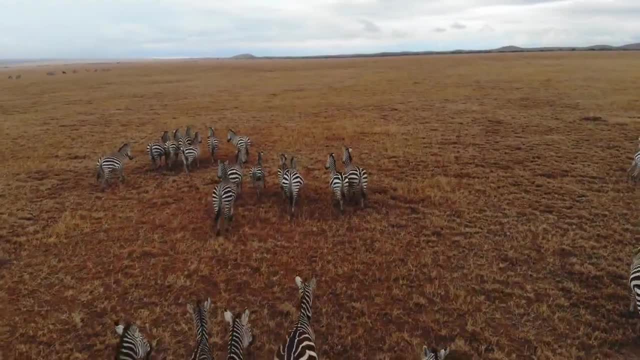 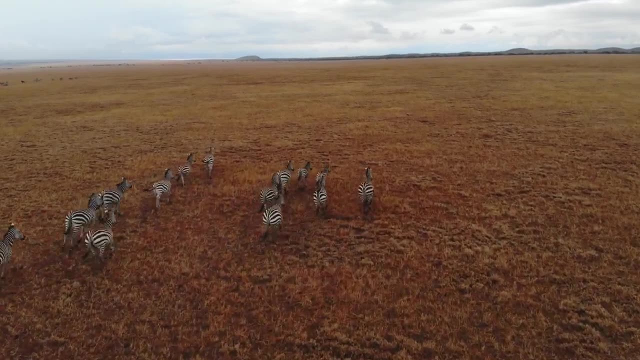 individual zebras. The lion has trouble picking out any one zebra, and so it doesn't have a very good plan to attack. It's hard for the lion to even recognize the zebra. It's hard to recognize which way each zebra is moving. 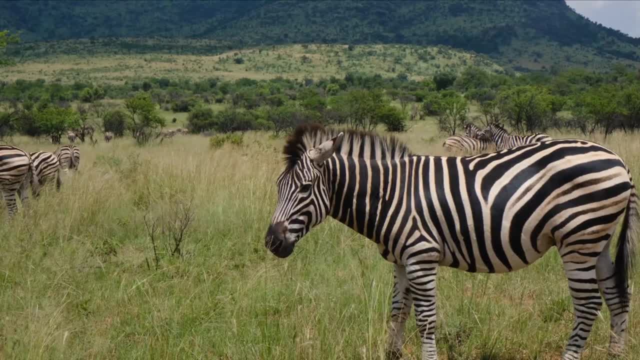 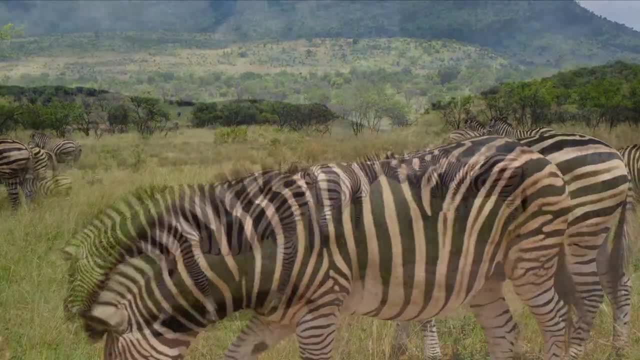 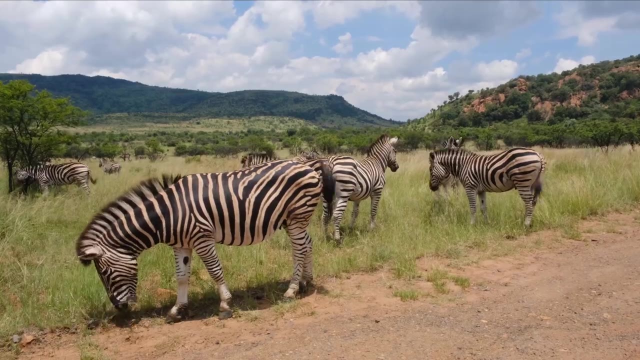 Imagine the difference between pursuing one animal and charging into an amorphous blob of animals moving in different directions. The lion's inability to distinguish zebras also makes it more difficult for it to target and track weaker zebras in the herd. Hope you enjoy this video and please do like and subscribe for more content in the future. Thanks for watching. 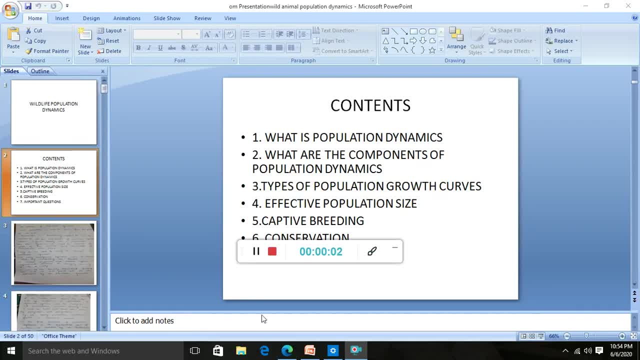 Hello and welcome to my next class, wildlife population dynamics. Well, it is actually not in continuation with genetic parameters and it's not genetic parameters part 3, as promised earlier. so I apologize for it, but it's for good, because this, the class of mine, is being put on population. 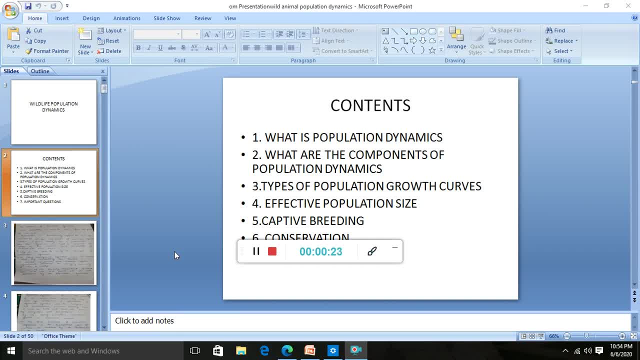 dynamics, wildlife population dynamics- solely for the students of my Mahirachi veterinary college, on demand of Mahirachi veterinary college, but meant for all of you who would like to see it online on youtube. Anyways, coming to the topic today which I have put it, I'll definitely be 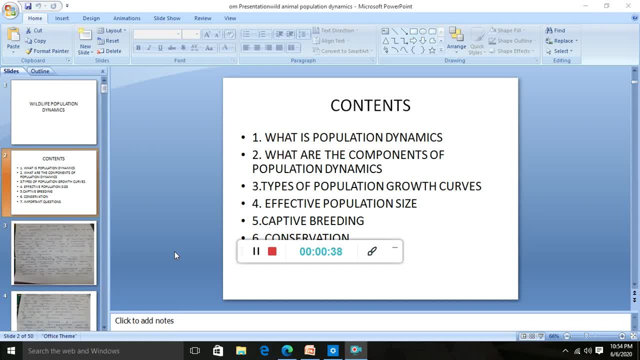 uploading genetic parameter part 3 soon for my students- Well, the students. the topic today I would be dealing with is wildlife population dynamics. So the content which I would be taking in this is: what is population dynamics? what are the components of population dynamics? 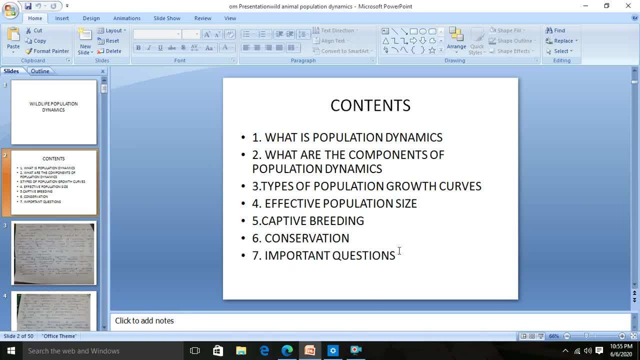 types of population growth curves, effective population size, captive breeding, conservative population size and so on. So the content which I would be taking in this is conservation and, of course, the important questions at last, which I try to do in every lecture of mine. Now, coming to the first screen, I think I should go for full screen mode now, for better.